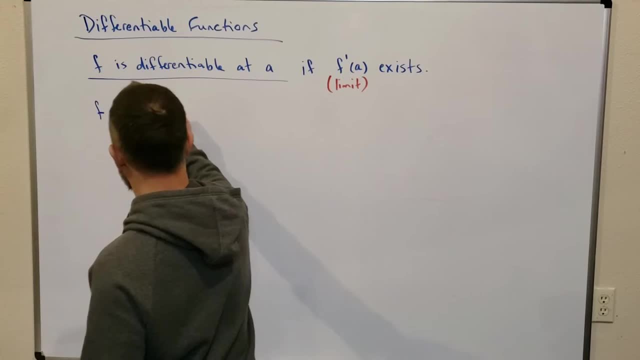 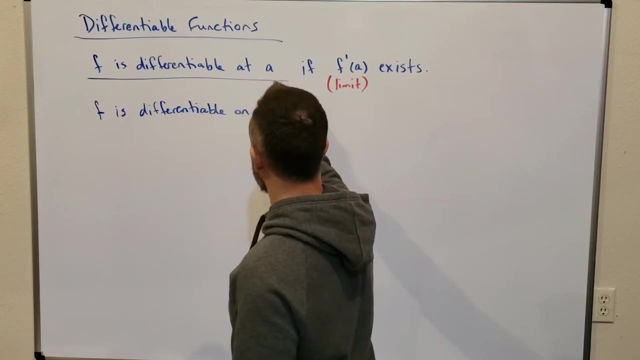 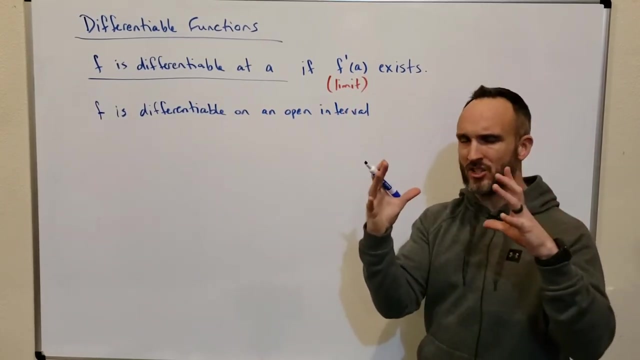 what it means to describe the f as differentiable. f is differentiable on an open interval. So an open interval is one with parentheses on each end. You don't include the end points. So we say: if f is differentiable on a number, it's giving you an idea of a number of puts in the box. So we say: 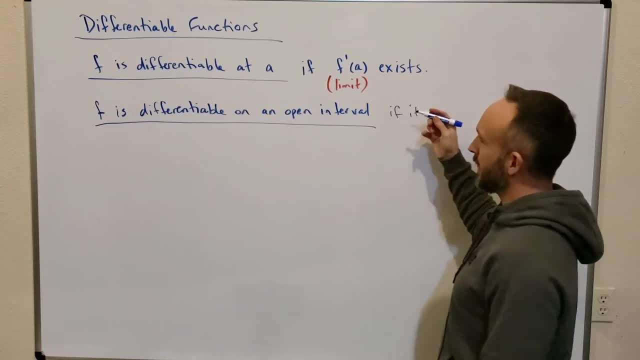 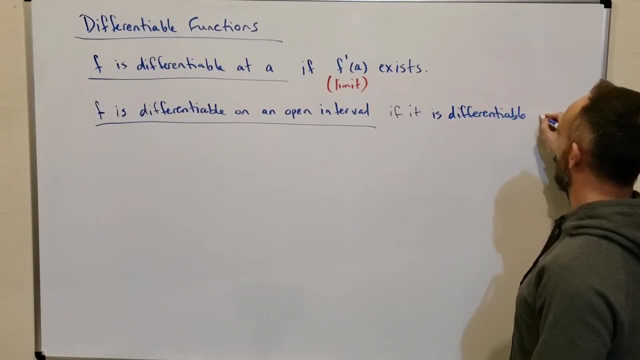 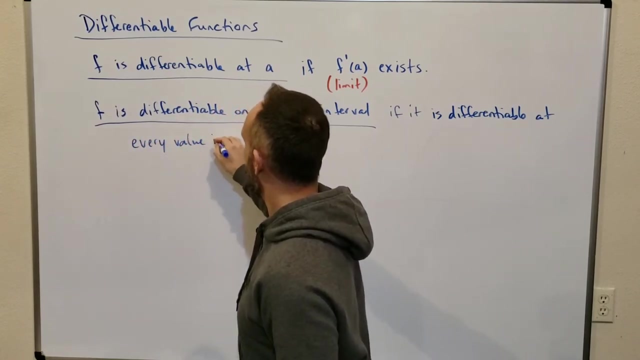 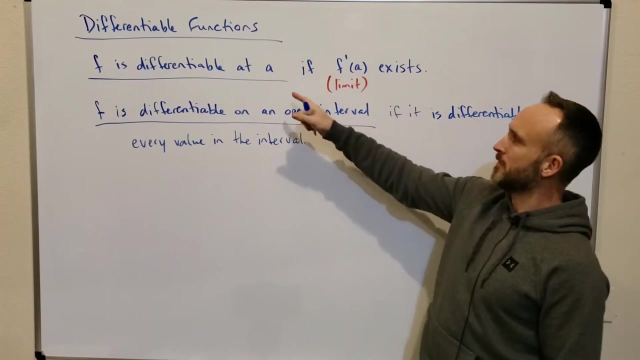 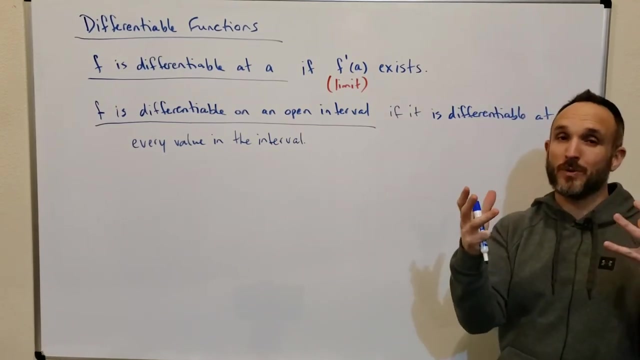 an open interval, if you could probably guess it. if it is differentiable, if it is differentiable at every value, at every value in the interval. okay, so we know what it means to be differentiable at a value. and now, if you get F being differentiable at values within an open interval, then we call it differentiable. 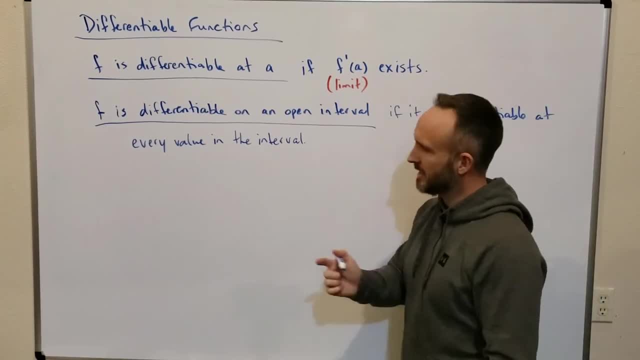 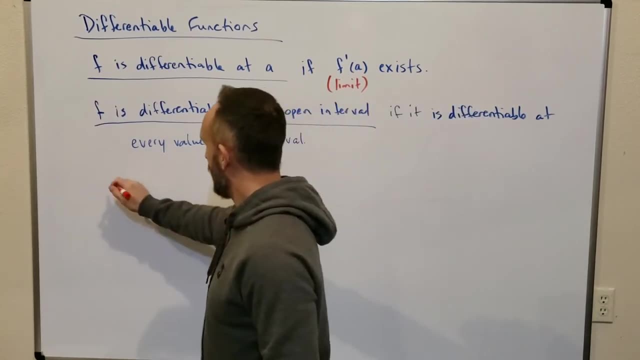 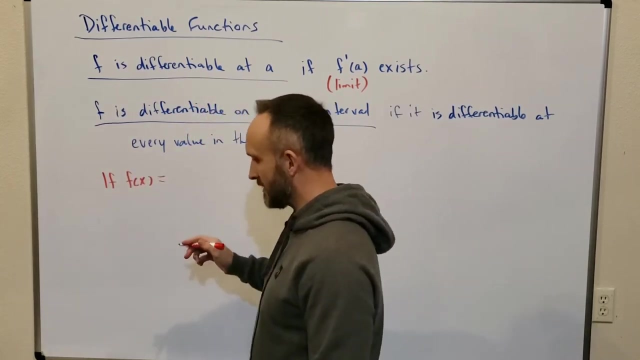 on that open interval. very simple, right so? so let's take a couple examples. let's use a different color here, so I'm not going to show why this is true. in fact, I just did it in a previous video. but if f of X equals 1 over X plus 1, then through. 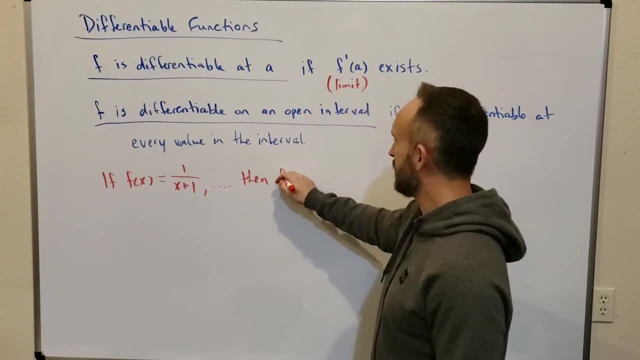 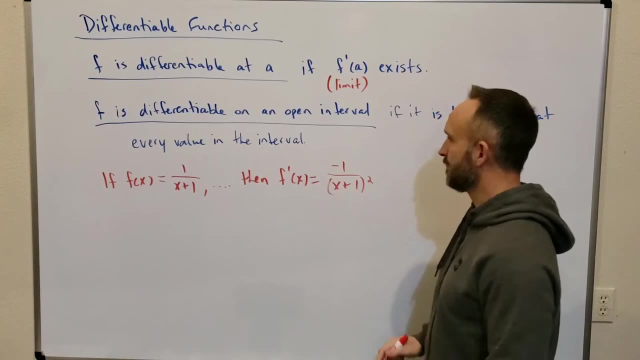 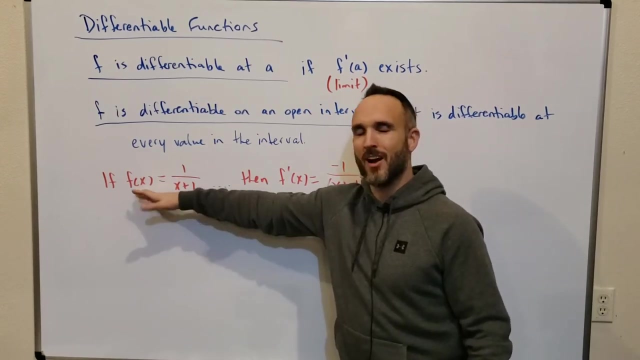 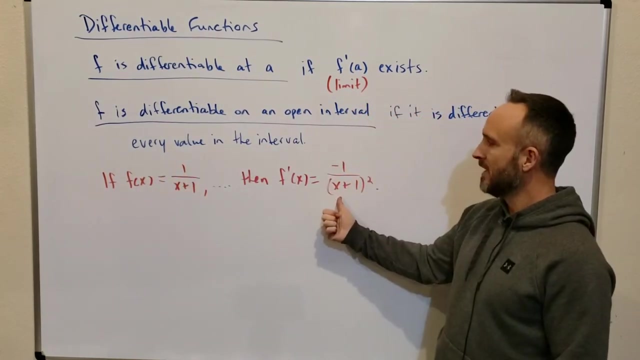 some work. you could see pretty quickly. the f prime of x equals negative 1 over x plus 1 squared. ok, so. so let's discuss the differentiability of the function f. well then, when you take the derivative of f, you get this formula and the function f. 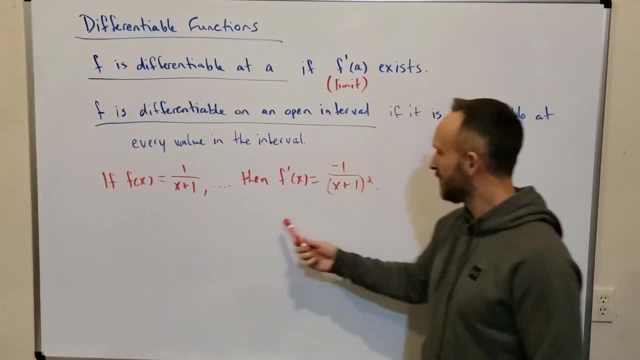 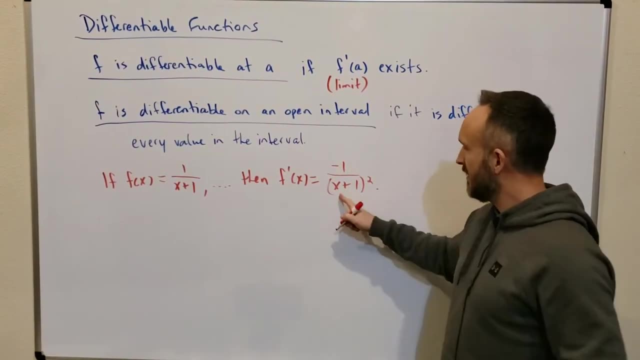 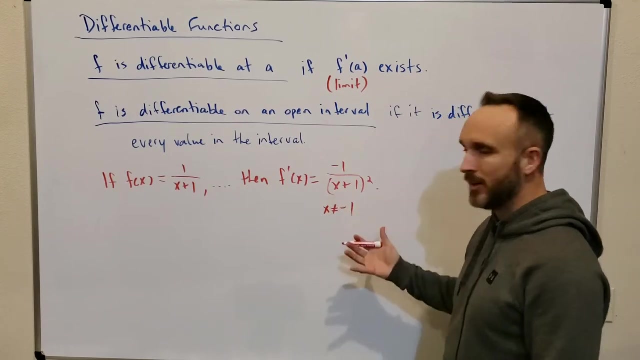 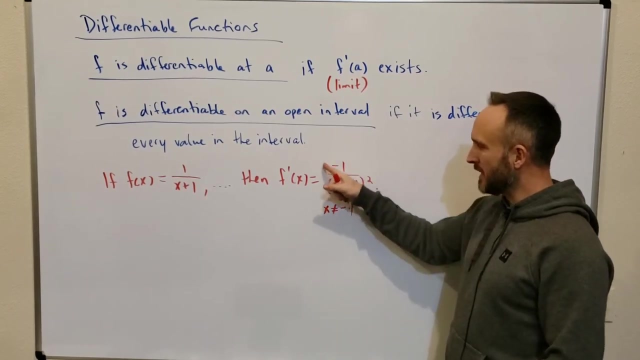 the function f is differentiable if this formula exists at that value. well, this, this formula can only be calculated. can only be calculated if x does not equal negative 1. right, if x is negative 1, you'd be dividing by 0. we can't do that, but any other value for x you could. 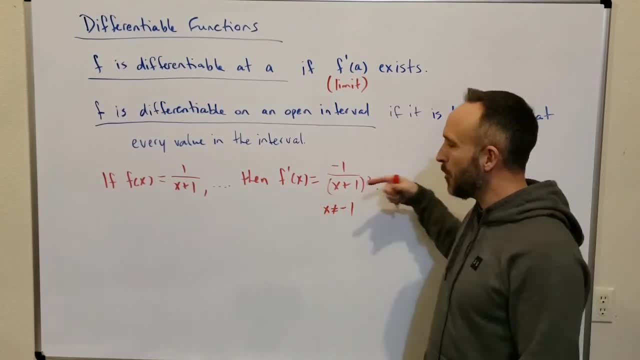 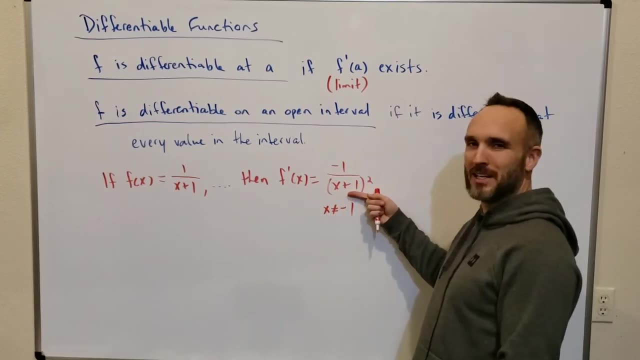 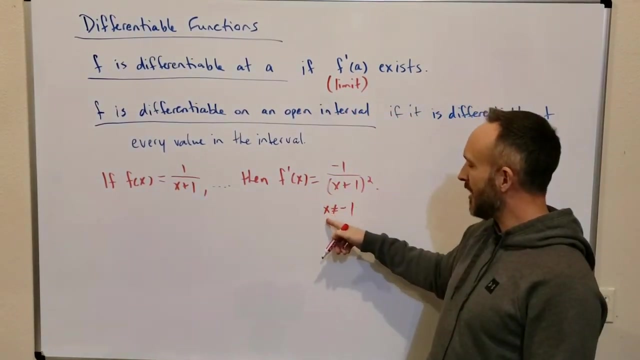 calculate the output of this formula. so we say here's, we go back, we see, we see when f prime can be calculated, right, We see when f prime can be calculated. and then we go back to f and we can say, well, since the derivative of f can be calculated here, we say that f 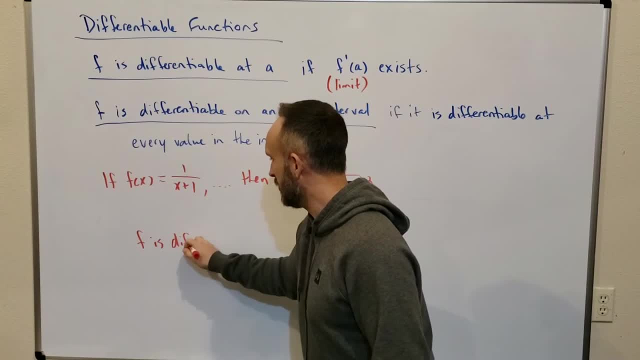 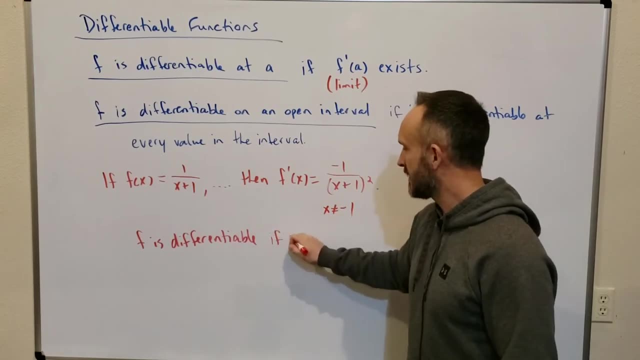 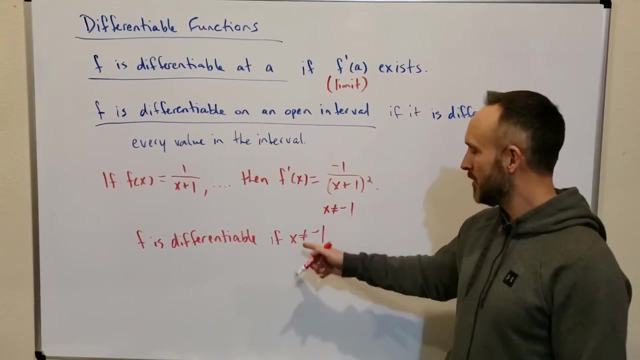 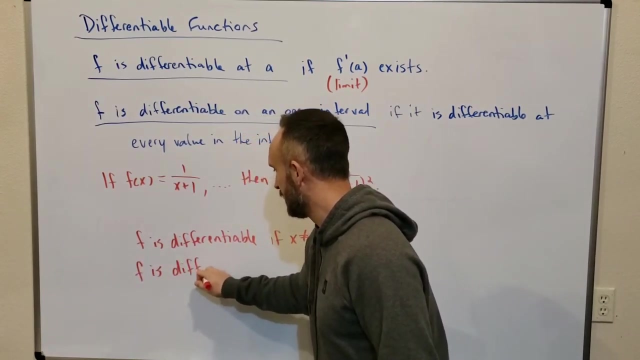 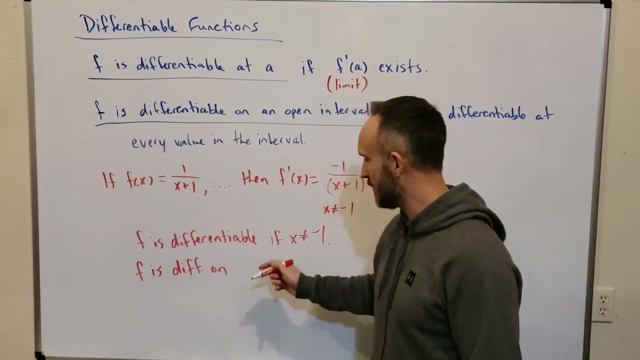 is differentiable if x does not equal negative 1. Any other x value f is differentiable. So typically what we do is use an interval notation. So we'd say f is differentiable on. when you go to intervals you say on, not at, or something like this. So let's say f is differentiable on the interval. 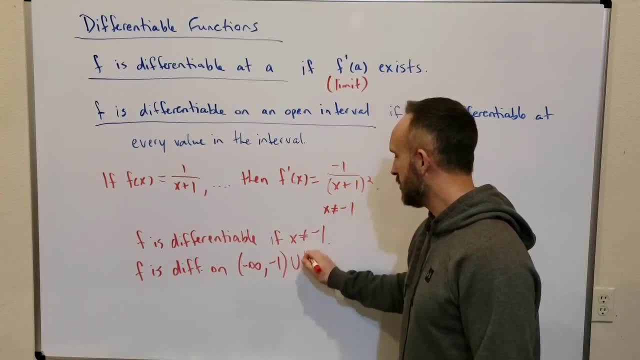 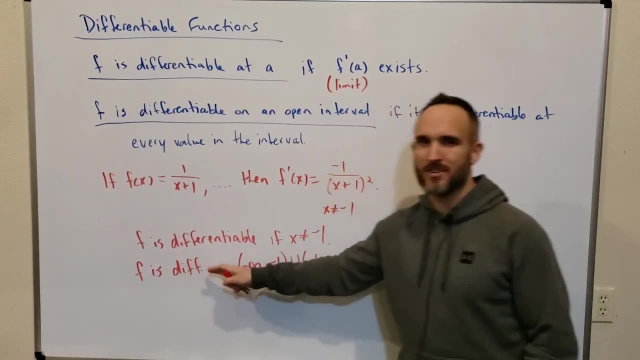 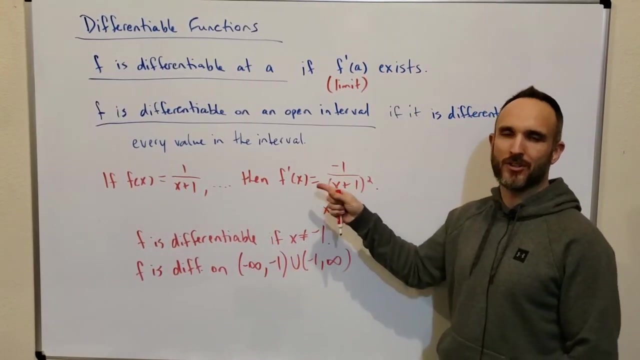 notation: Negative infinity to negative 1, union negative 1 to infinity. okay, So notice that I don't say f, prime is differentiable. F is differentiable because of properties exhibited by the derivative of that function. So it's really important when you start learning this, when you start working. 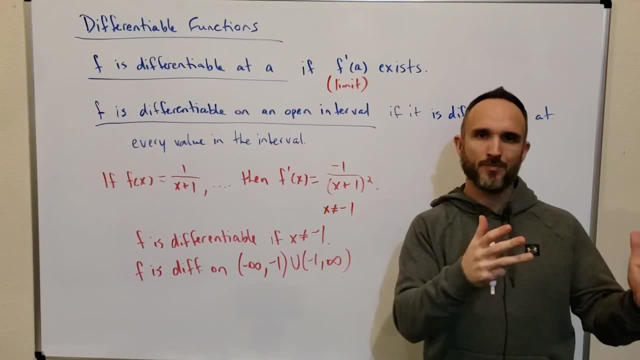 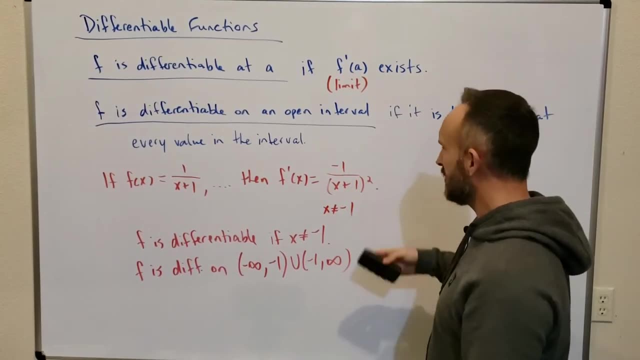 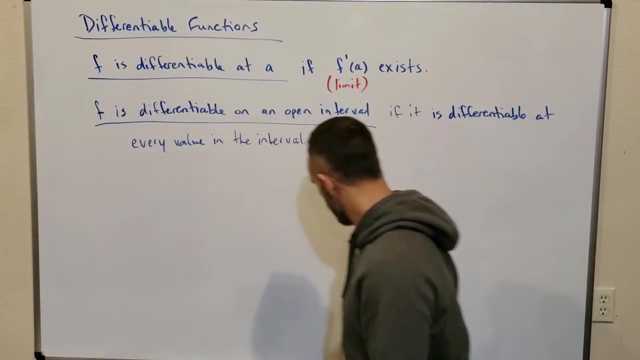 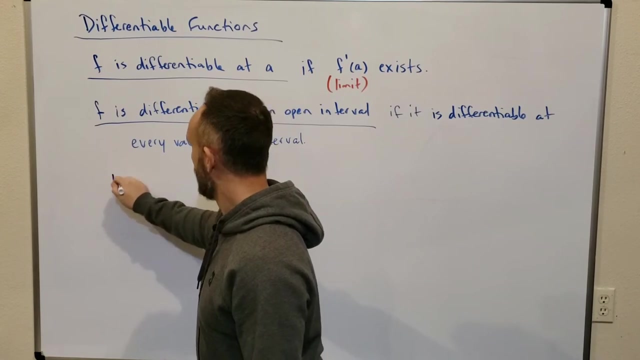 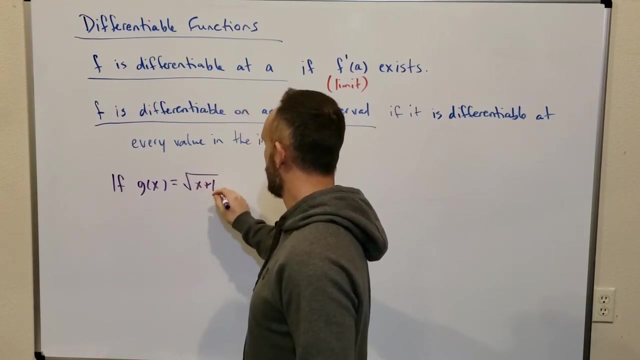 with it to really distinguish between f and f prime. If f prime exists, then f is differentiable. So make sure you get a handle on that. Okay, Let's try another one similar to this. Let's suppose g of x equals the square root of x plus 1.. Again, through some work you could find. 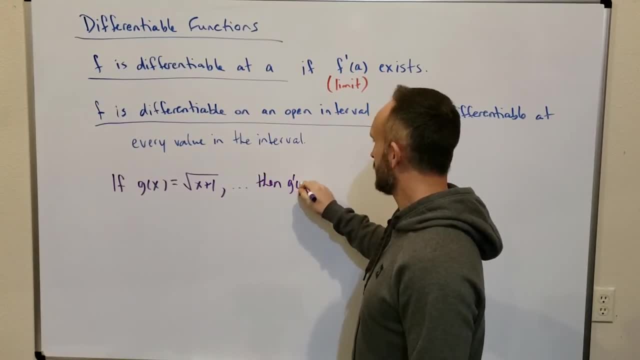 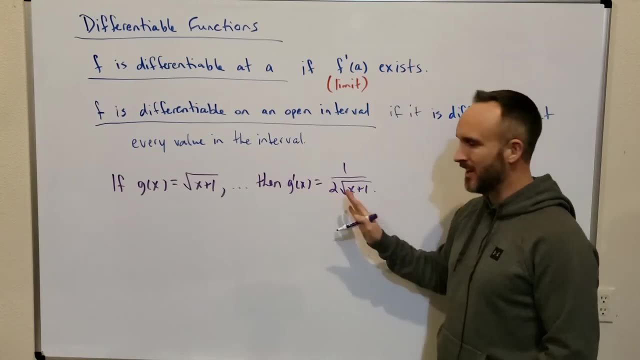 its derivative and you could say that g prime of x equals 1 over 2 times the square root of x plus 1,. okay, This video is not about how to calculate that. It's just about discussing the differentiability of functions. Well, this function. 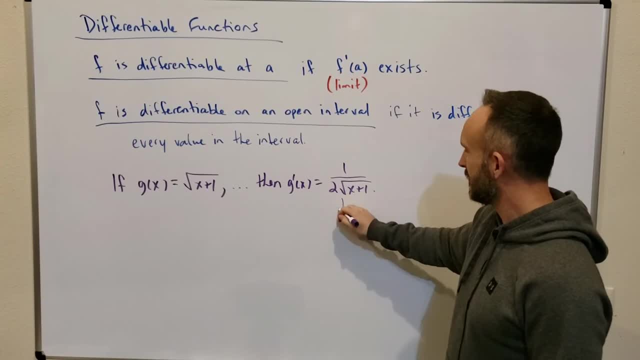 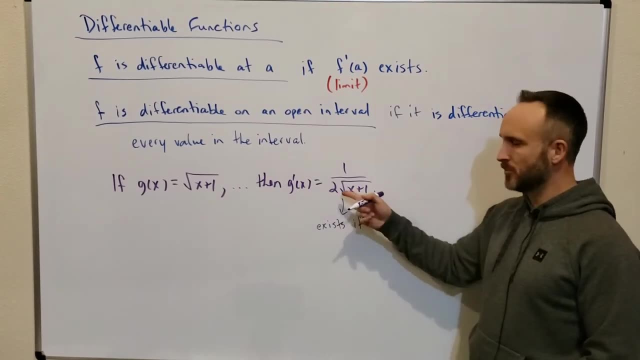 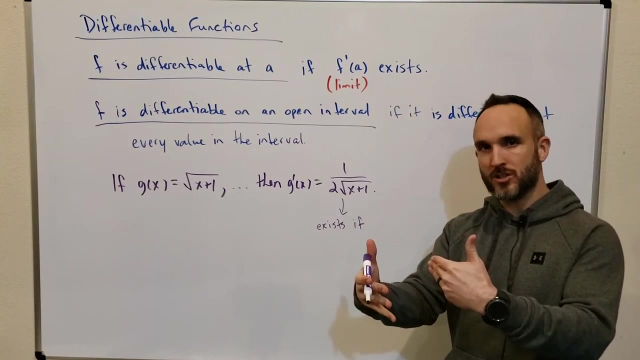 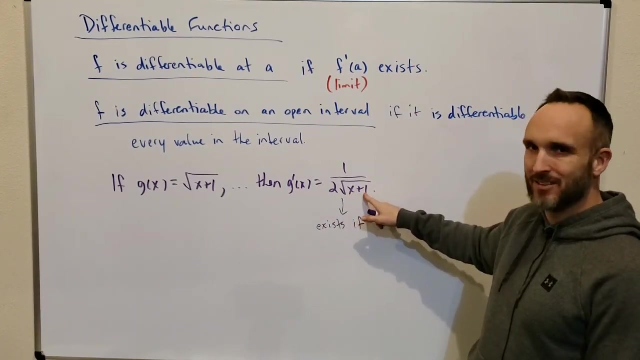 the g prime of x function exists. this guy exists. Well, clearly, x can't be negative 1, because we'd be dividing by 0. But also x can't be numbers smaller than negative 1,, like negative 1.2,. right, If x were negative 1.2, and you plugged it in: negative 1.2 plus 1 is negative. 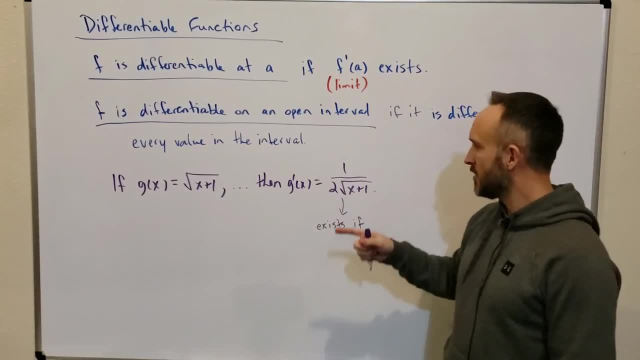 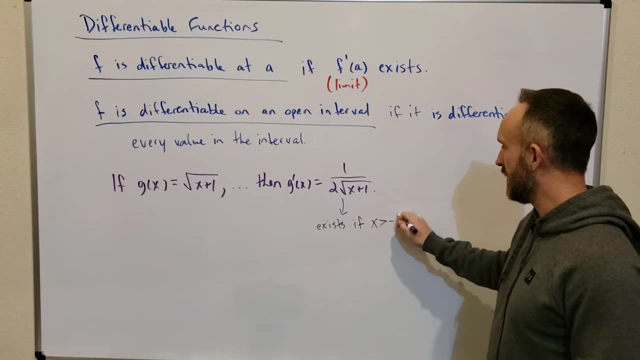 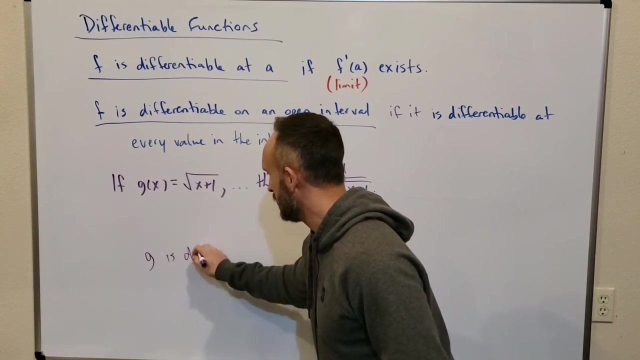 and the square root of a negative number is an imaginary number. So x can't be negative 1, or anything to the left of negative 1.. So x has to be greater than negative 1.. So we say here the function g is differentiable. Let's go right to the interval notation. 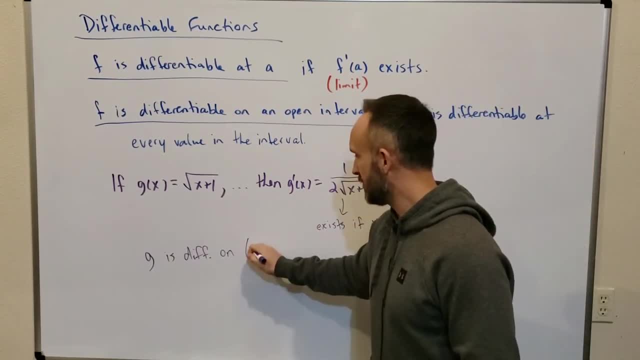 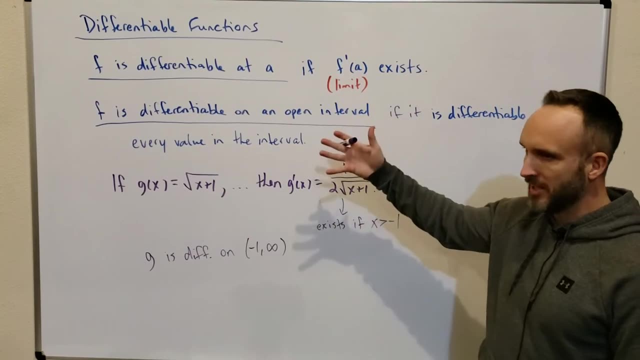 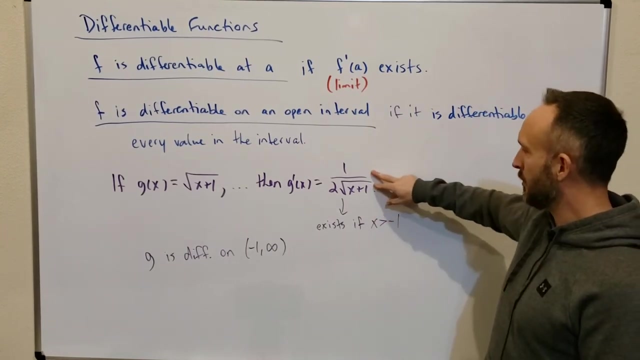 The interval notation for everything bigger than negative 1 is parenthesis, negative 1, comma, infinity. okay, So this video is all about understanding differentiability, which of course takes into account the derivative function itself, And basically being able to find the domain of the derivative. you have to understand when this value exists. 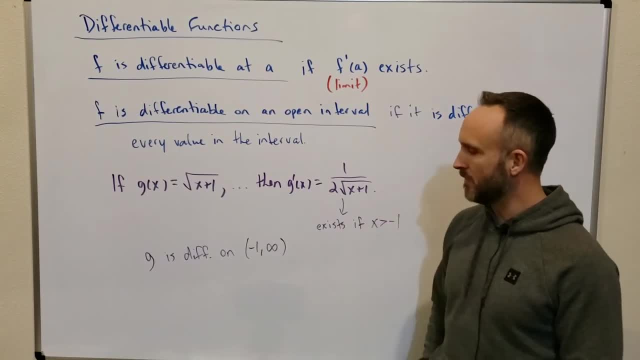 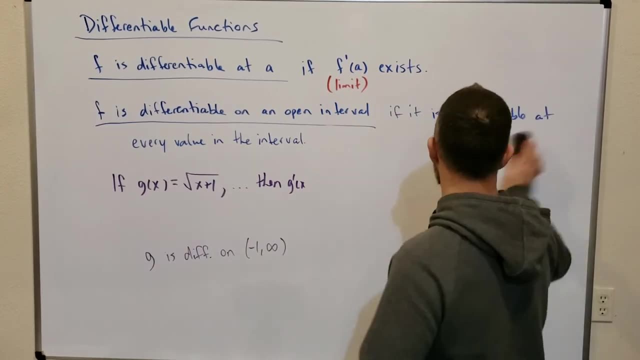 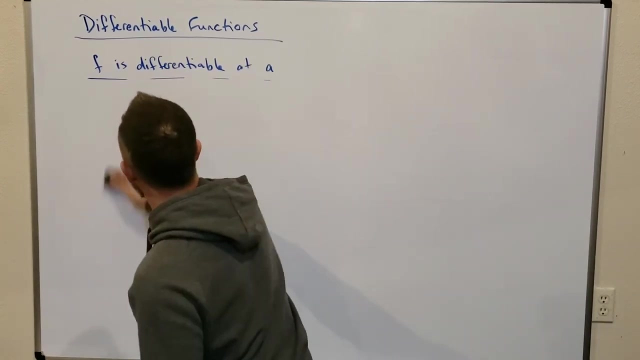 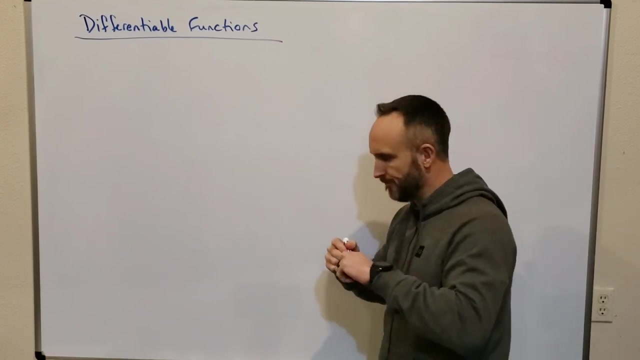 You have to find the x values for which this value exists, to determine where a function is differentiable. one really cool thing about this differentiable property is the following theorem, And you don't want to get this backwards, Okay, So this is really important. 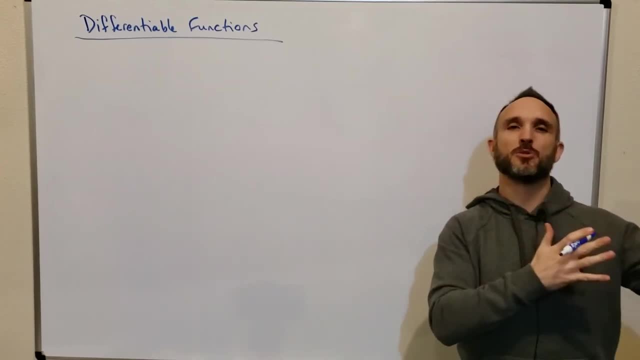 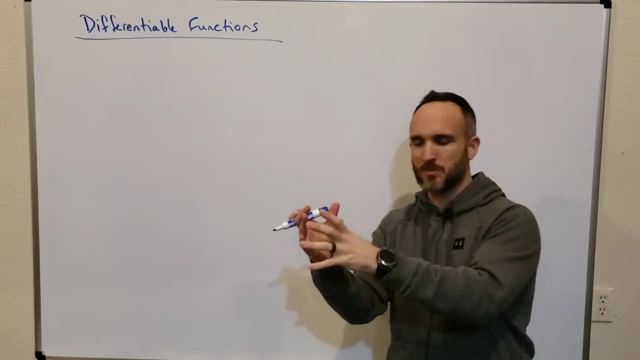 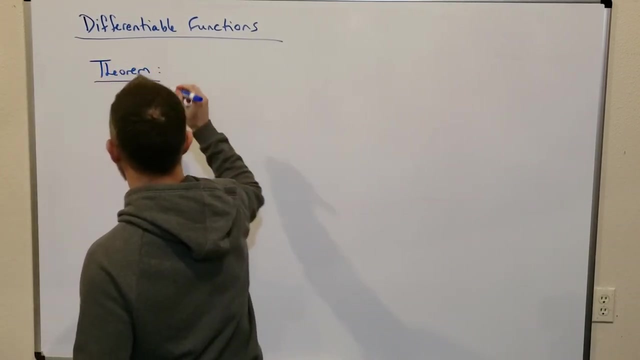 We looked at continuity of functions and now we're looking at different ability of functions. The differentiable part is actually more, more strict than the continuous part. Okay, So that can help you kind of remember this theorem. This theorem says: if F is differentiable, 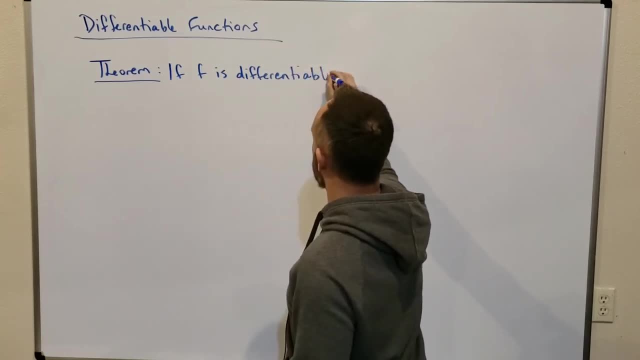 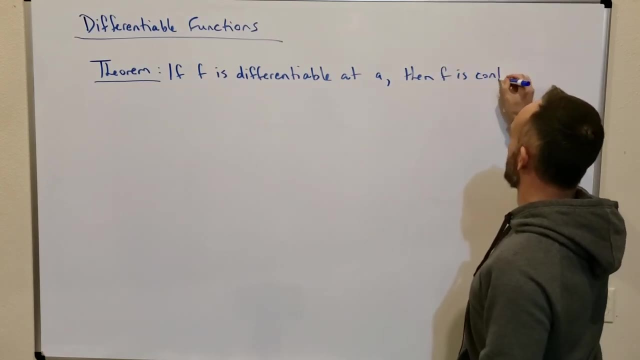 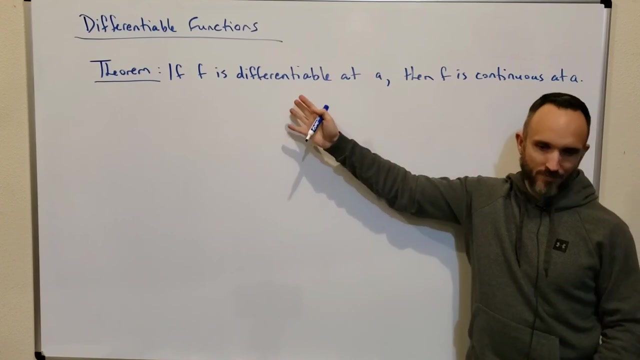 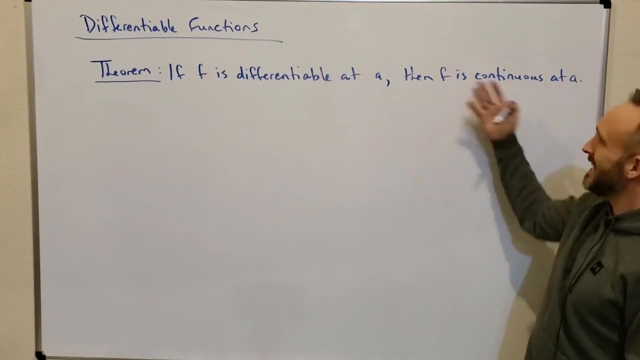 if F is differentiable at a value a, then F is continuous at a, So differentiability is a sufficient condition for continuity. If F is differentiable there, it has to be continuous there. But it's not always true that a function. 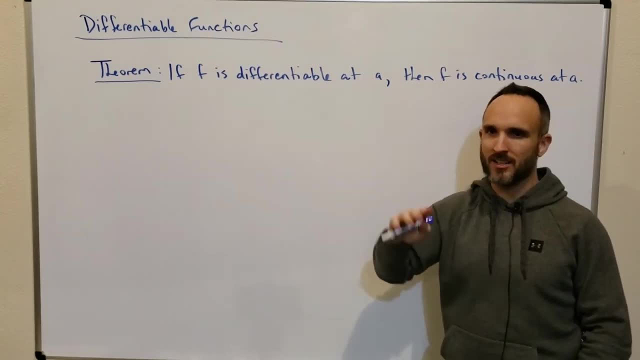 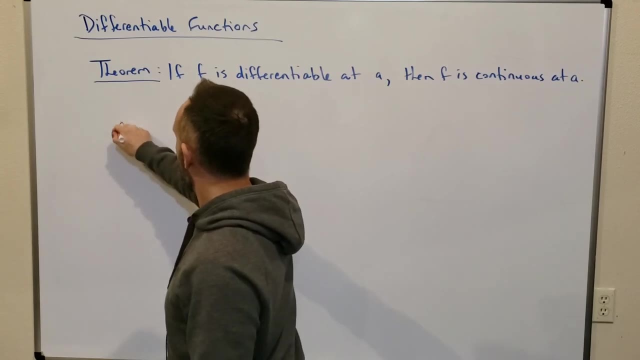 if a function is continuous, it is also differentiable, So that's not enough. Okay, However, if we look at what's called the contrapositive of this. So if you take further math, you'll see this in future classes. 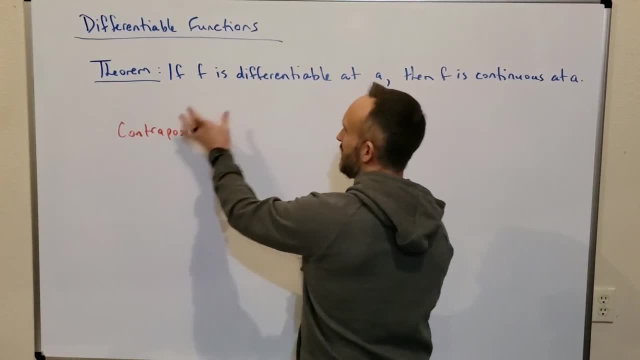 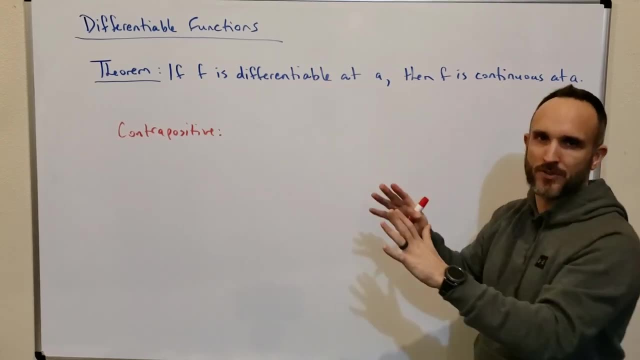 But the contrapositive guarantees that if you have an if-then statement, you can reverse it if you make both of these conditions opposite of what they are. That's a very rough description here, So the contrapositive has to be true also, which would say well.